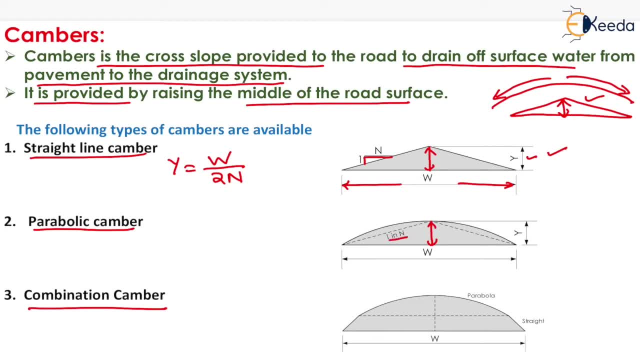 is Y and slope is one in n, which is written here, and the overall width is W, which is written here. So we can compute the value of Y, which will be equals to W, which is equal to 2x, square upon n, W, and that is the profile of combination. 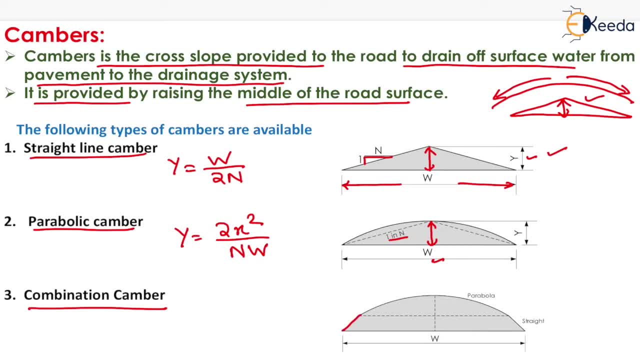 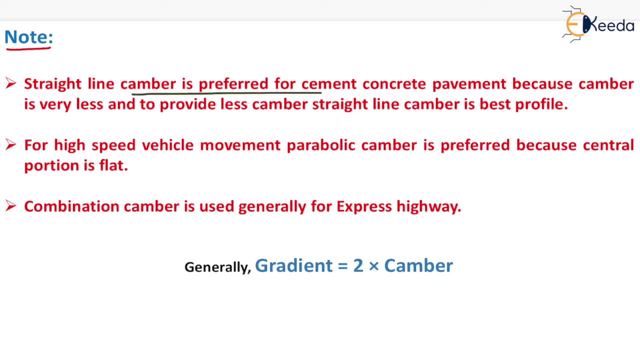 camber. in the starting straight line camber is provided just like this and in the middle portion parabolic camber is provided, So it is combination camber. Now note is written here that is straight line camber is preferred for cement, concrete pavement because camber. 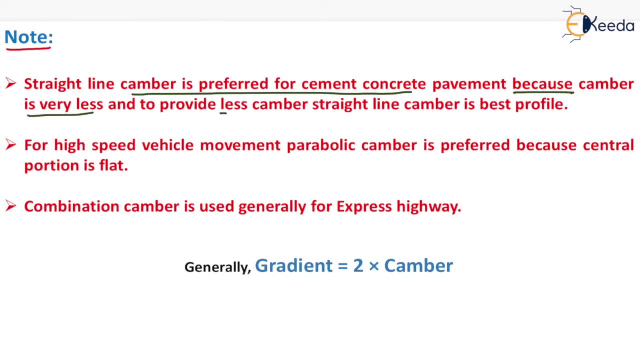 is very less in case of rigid pavement, provide less camber. straight line camber is the best profile. so to provide very less camber in a rigid pavement, the straight line camber is the best profile. that's why straight line camber is generally preferred for cement concrete pavement. 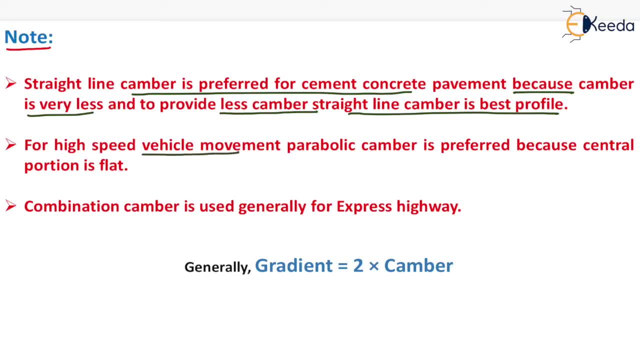 now for high speed vehicle movement, parabolic camber is preferred because central portion is flat. now, in parabolic camber central portion is generally flat. that's why it is generally preferred for high speed vehicle movement. now, combination camber is generally used for express highways. now if we want to determine the gradient then it will be equals to two times of camber. now we have 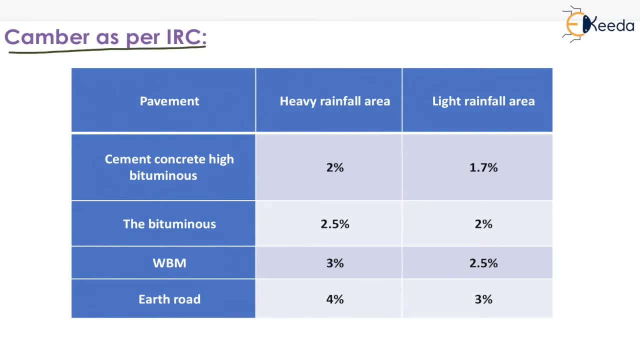 the camber. as per indian road congress for heavy rainfall area and for light rainfall area. as per indian road congress for heavy rainfall area and for light rainfall area area. now in the first column, pavement is written, and here heavy rainfall area and light rainfall area is written. now for cement, concrete or high bituminous pavement in case of heavy rainfall area. 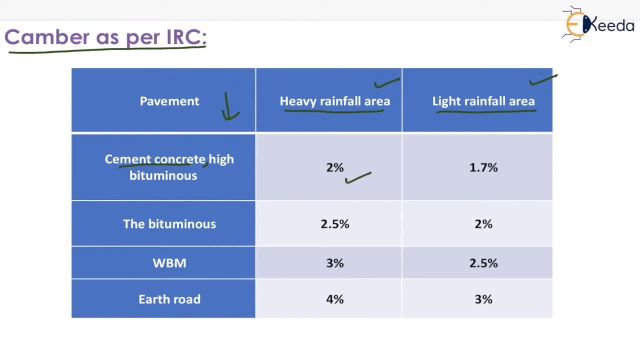 the camber is 2 percent, and for light rainfall area, the camber is 1.7 percent. now for thin bituminous pavement: in case of heavy rainfall area, the camber is 2.5 percent and for light rainfall area, the camber is 2 percent. for water bound macadam: in case of heavy rainfall area, camber is: